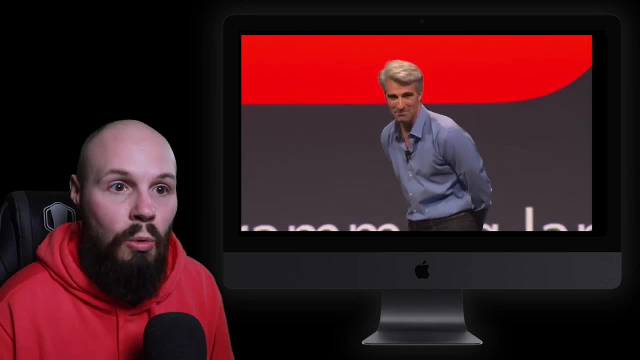 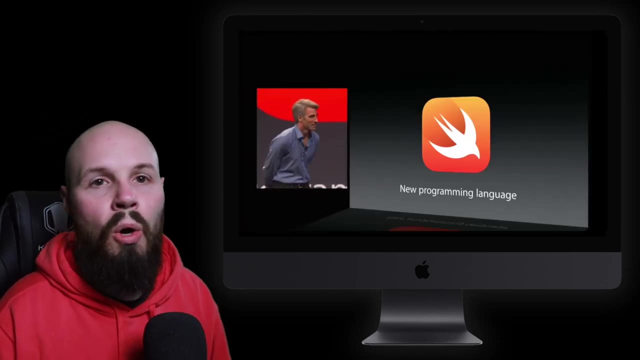 Like developers had no clue it was coming. they were watching the announcements and it's like holy crap, a whole new language. Like everything changed back in 2014 when Swift was announced. What the engineers at Apple did was they took all their previous knowledge with Objective-C and everything. 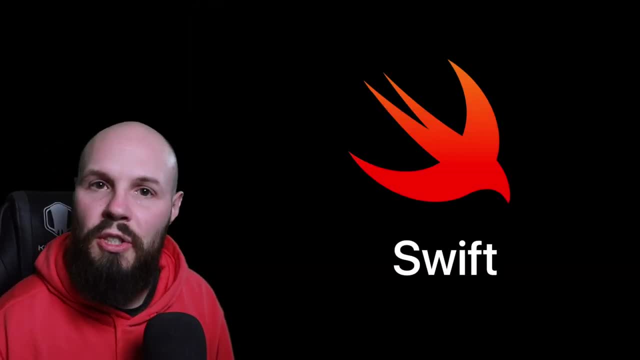 because Objective-C is, you know, 30 years old and they did all their research on the new and modern languages and where things were going and they took all that and they built Swift, Apple's next generation programming language that is for their future. 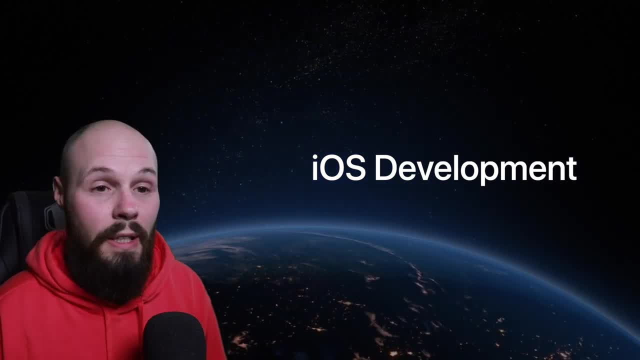 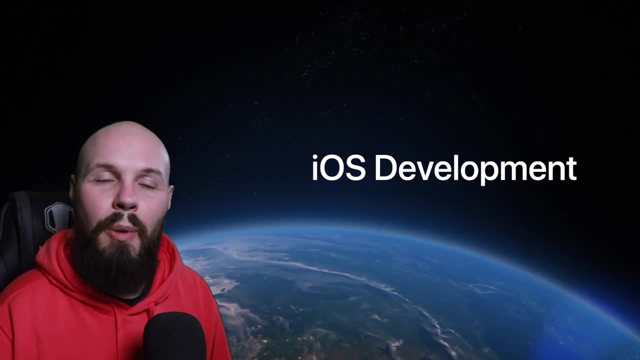 Now a lot of people always ask me: you know, because native iOS development? admittedly it is a niche programming language. It's not as widespread as you know Java or JavaScript or Python, But it is niche. so a lot of people ask me, like: if I become an iOS developer, like, does that limit my career choices? And I always say, like, as a Swift developer, iOS developer, whatever you want to call it, you're tying your career to Apple And as long as you believe that Apple's not going anywhere and it's going to be around for a long time, you know, into AR, VR, whatever direction they go. 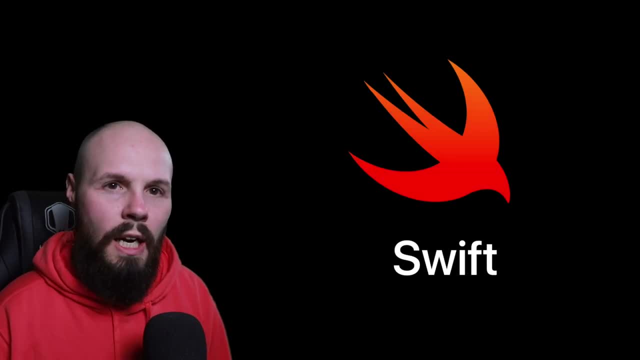 I think that's a pretty safe bet. Speaking of safety- amazing segue- one of Swift's major selling points is it's just a safe language. There's type safety Objects, you know can't. It can't be nil unless you use optional. 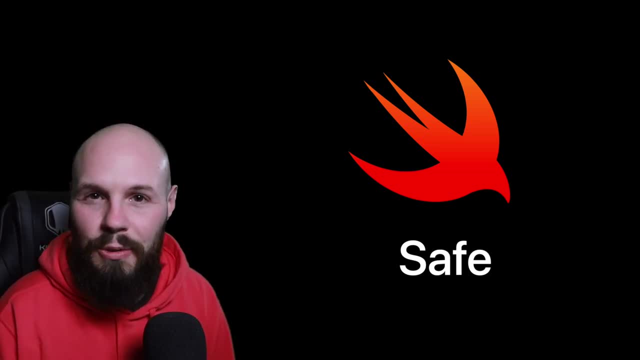 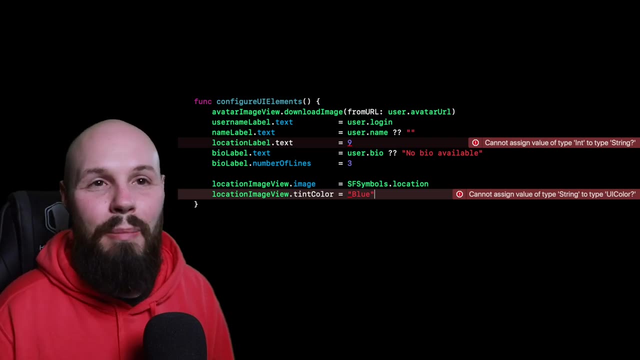 Basically, a big thing of Swift is you want to have a lot of compile time errors, not run time errors. As a new programmer, newly aspiring programmer, that may have meant nothing to you. Basically what that means is Swift tends to give you errors at the time of writing your code or when the code compiles in Xcode. 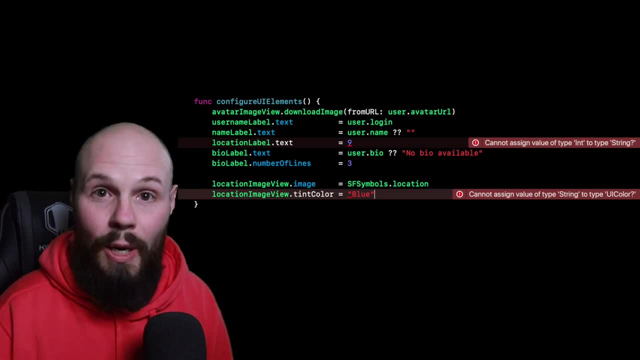 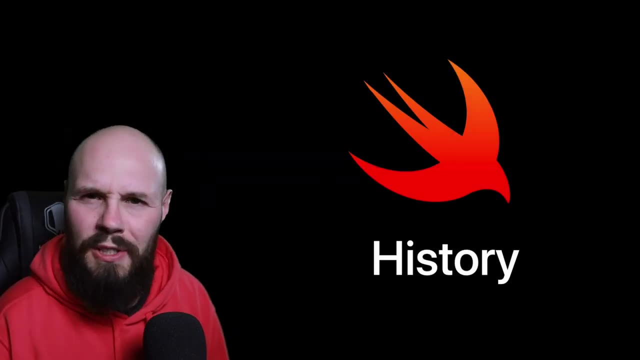 Whereas run time errors are. you don't know about the error until the app crashes. Then you got to debug, So you're going to see a lot of compile time errors before you can even build your app with Swift. Let's run through Swift's very brief history. 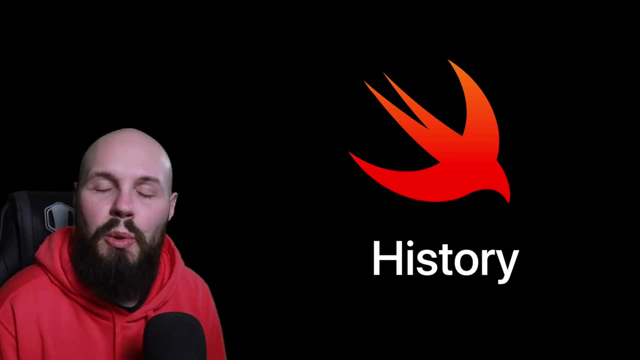 Again, it was announced in 2014,. just to let you know, kind of, how Swift has evolved over the past couple of years Now. Swift had some massive changes, and very rapidly in its early days, And the reason you should know this as a new beginning Swift developer is because if you look for a blog post or maybe a stack overflow answer or some resource that is old and hasn't been updated since, you know, 2015,, 2016,- that can get you in a lot of trouble. Because again through 2014,, 15,, 16,, 17,- Swift has changed A lot, but the good news is that change is starting to slow and Swift is slowly starting to mature. All right back to the beginning. 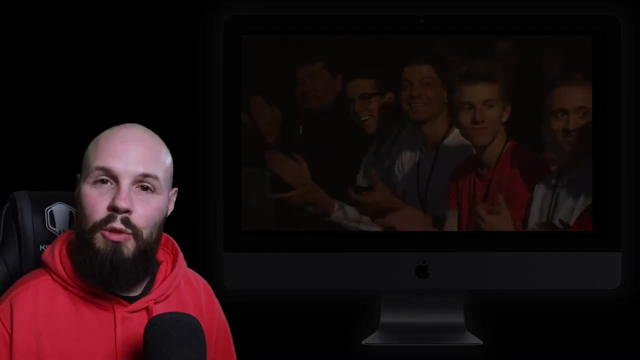 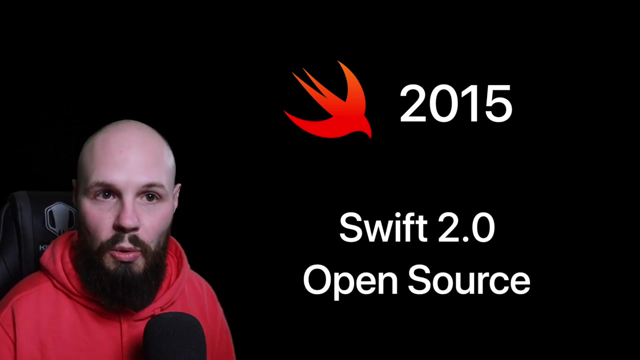 Like I said before, it was a surprise announcement in 2014. by 2015, Swift 2.0 was announced and it was also announced that WWDC in 2015 that Swift was going to go open source later that year and ended up going open source and Swift 2.2 later, like in December of 2015.. 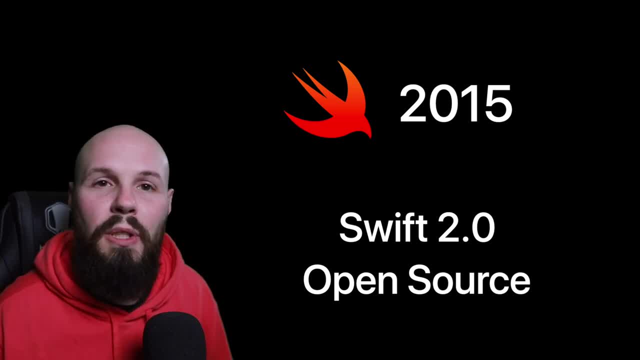 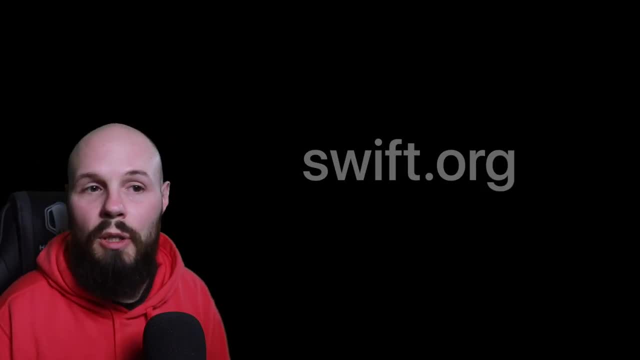 Now, open source was a big deal because that meant the iOS developer community as a whole could contribute to Swift language. If you ever want to look into this, go to swiftorg. You can see the forums and see the discussions on proposals that are going to be implemented into Swift. 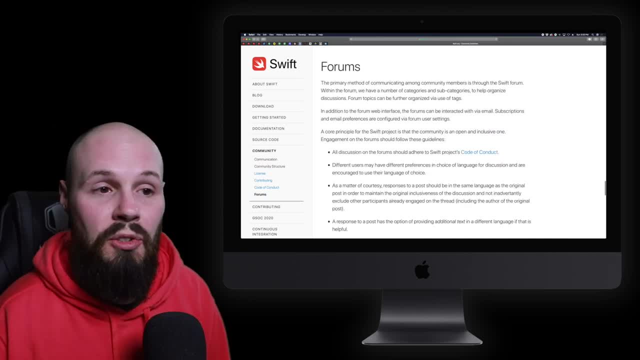 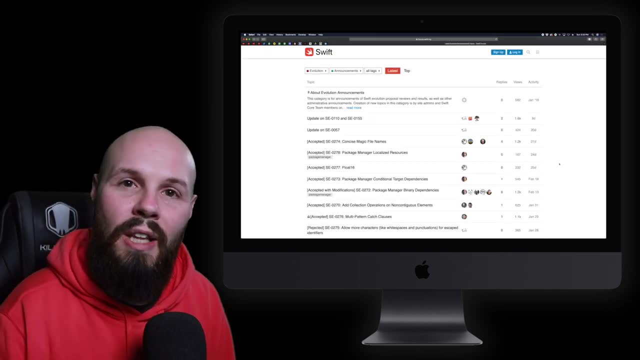 Now don't get me wrong, This is like heavy language implementation details. Most of it's even over my head. But if you are interested in like how the language gets built or you know what new things are coming to the language, that's a spot to go look. 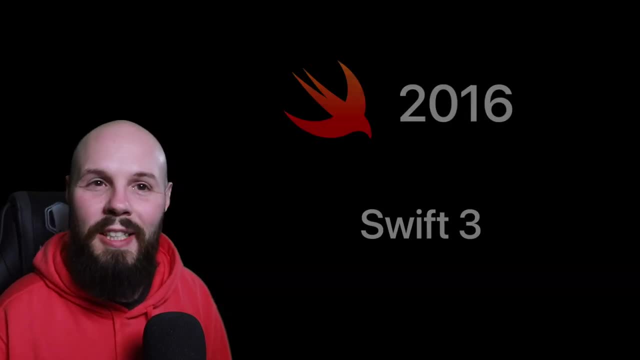 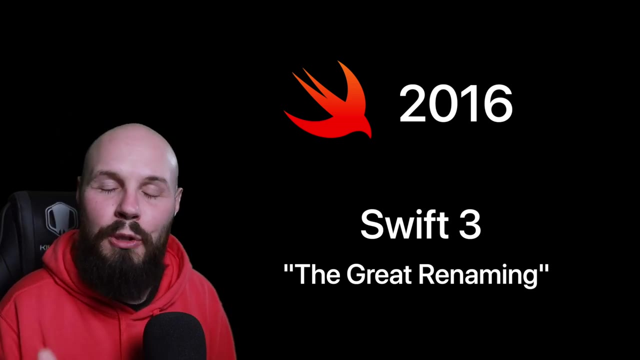 Now going open source was a big deal, But in 2016, Swift 3 came out and that was a huge deal. That was dubbed the great renaming. Basically, what happened between Swift 2 and Swift 3 was a ton of breaking changes in Swift's API. 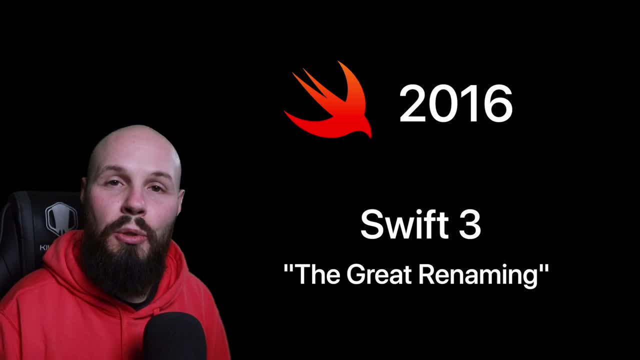 So it was a nightmare converting a Swift 2 codebase to a Swift 3 codebase, because so much broke and so much changed. However, Swift 2 to Swift 3 was kind of like just ripping off the Band-Aid right. 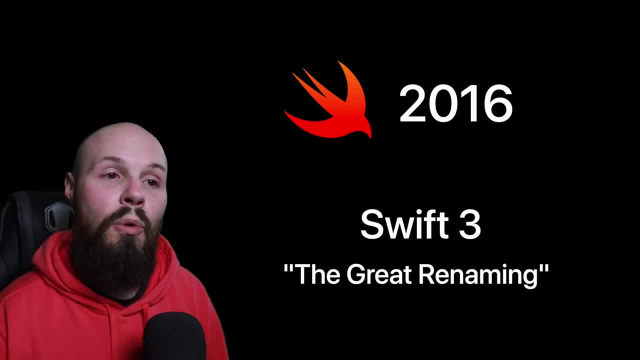 It was a ton of pain right there. But you know, Swift 3 to Swift 4, Swift 4 to Swift 5 and upcoming Swift 5 to Swift 6 have been a breeze compared to that, So they kind of got all the pain. 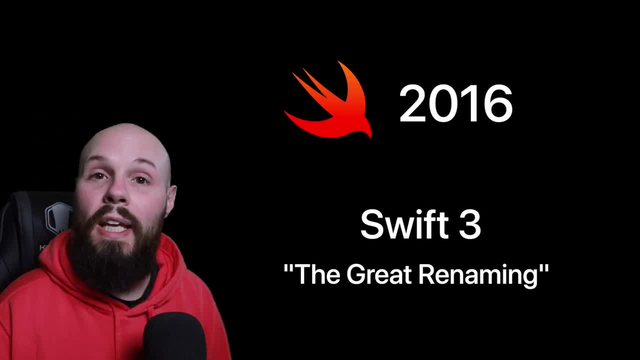 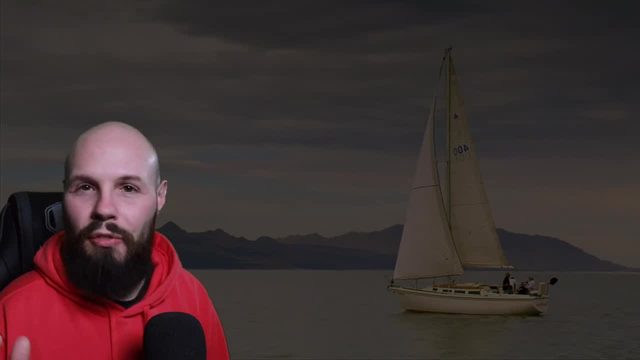 All the pain out of the way going from Swift 2 to Swift 3.. So again, when you're looking at old resources or old blog posts, if it was done in Swift 2, stay away from it. But, like I said, after that major Swift 3 pain, it's been smooth sailing since then. Swift 4 came out in 2017.. But Swift 4 kind of was the last major number release at WWDC. Up until Swift 4, again, every dub-dub, which was June of every year, we would get a new Swift. 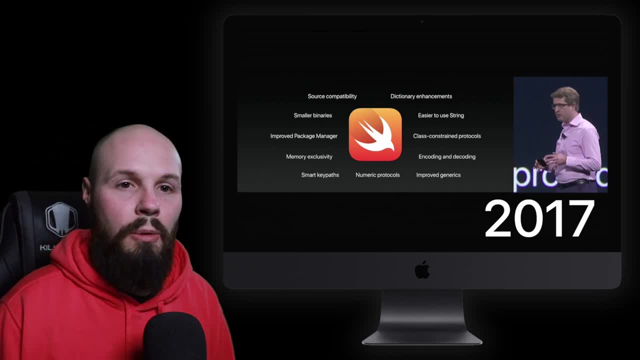 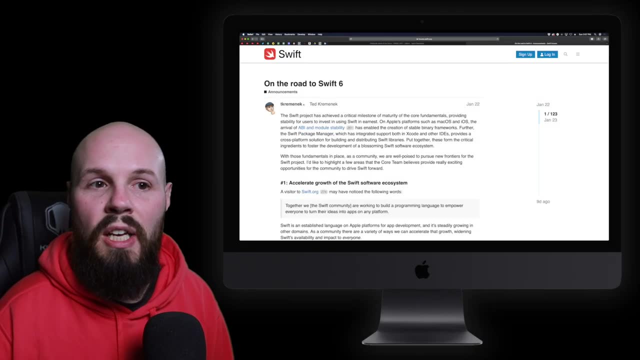 Swift 3, Swift 4.. Well, they've kind of slowed down since then And you know, WWDC 2018 was Swift 4.2.. It has slowed down And they recently announced on the roadmap to Swift 6 that you know there's no major year release. 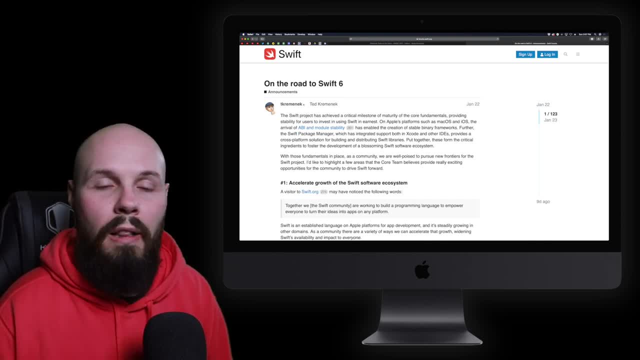 It's just going to release when it's ready, which is great. I love that, because it almost felt like they were rushing features into the language to make the annual release cycle. And you know, they've kind of learned and said: you know what? Swift 6 will release when it's ready. No release date It'll come Again. that, Along with the fact that you know the changes coming aren't major breaking changes, shows that the language is maturing And because the language is maturing, we're starting to see it leak out into non-Apple native platforms. 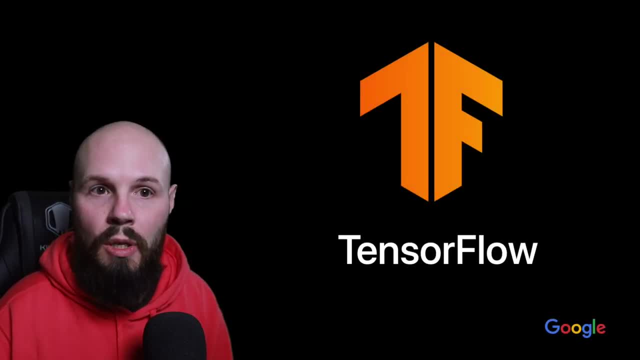 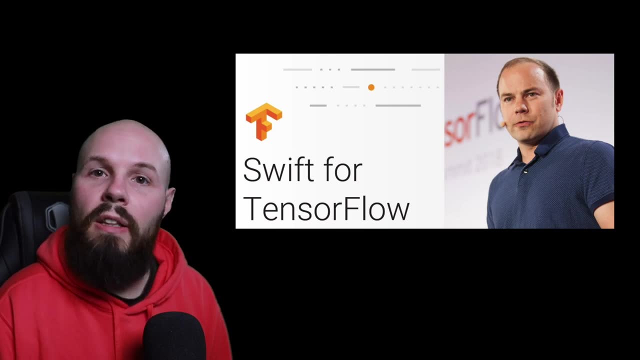 For example, machine learning at Google via TensorFlow. that is done in Swift. now, That's in part to Chris Lattner, who is one of the main developers behind creating and launching Swift at Apple. He had left for Google and brought Swift over to TensorFlow. 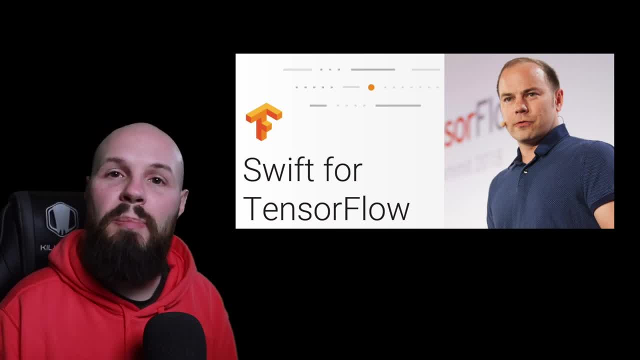 He has since left Google as well- just recently- But he was spearheading Swift. He's also spearheading Swift at Google as well, So you know it got a good foundation over there And now you can also write server code in Swift. Swift is almost ready for Windows. That's being actively worked on. But again, Swift is such a young language that you know it may not be on all these other platforms yet, But you can start to see the beginnings of it And if you kind of fast forward your mind five to ten years, it's looking pretty good. 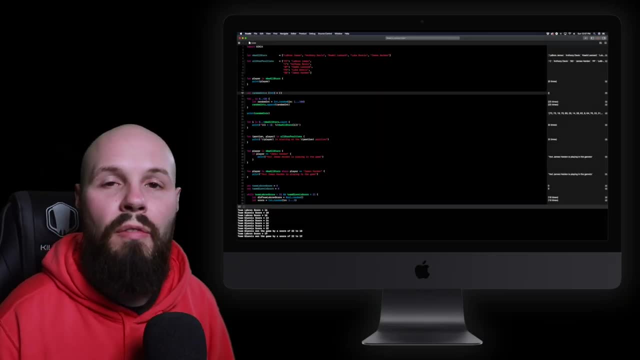 Now we're about to go into a bunch of videos about the basics of the Swift language. I want to reiterate that these are just highlights. These are just high-level videos. right, A lot of these topics could be almost whole courses in and of themselves, or at least multiple 10, 15-minute videos. 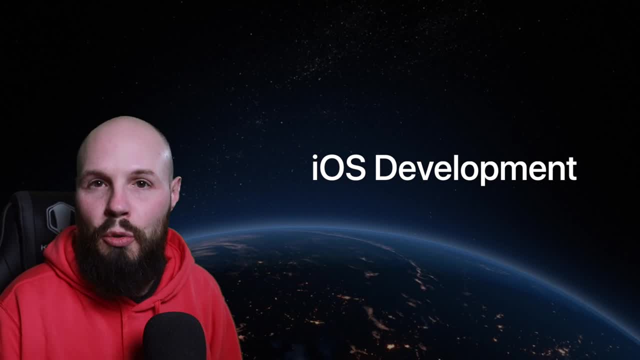 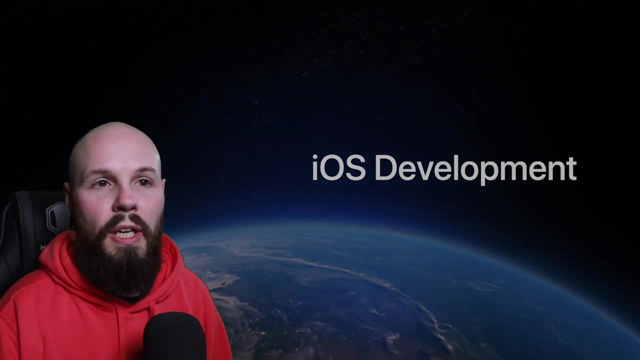 Again, like I said before, this is supposed to be your first video, just your exposure to this world. So, again, these topics will be pretty high level, But it is a good foundation for your future learning. Speaking of future learning, I want to recommend a couple of resources for you to check out to again just expand your world of Swift. 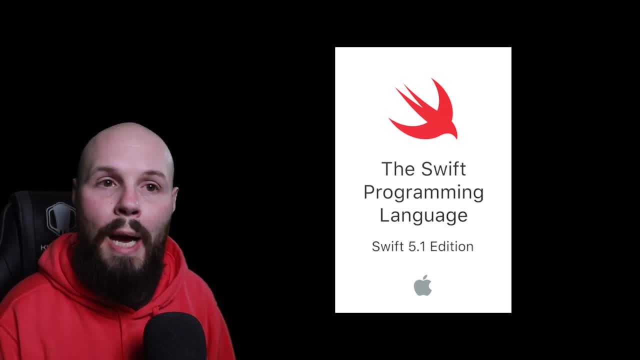 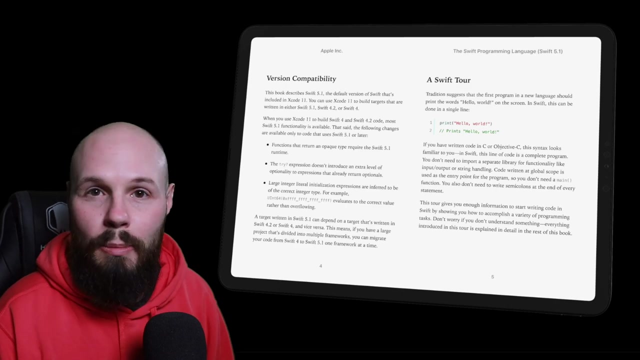 First is the Swift Programming Language Book directly from Apple. A little bit of a warning, and we're going to talk about this later in the books video, But this is basically Apple's instruction booklet for Swift, So it is pretty technical. I remember reading it as somebody who had never coded before and just started my Swift journey, which may be exactly where some of you are at. 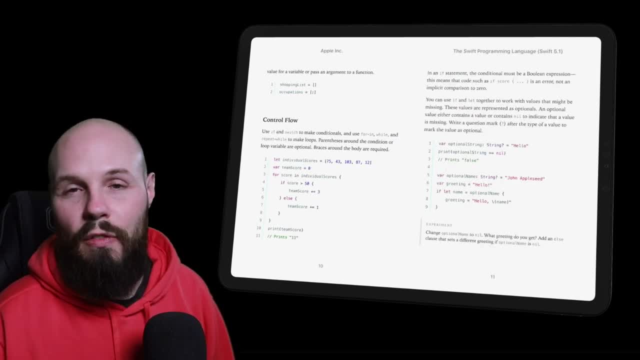 It was way over my head, But it is a very valuable piece of information. So I do recommend at least checking it out. But again, don't get discouraged if you don't get any of it. It's a pretty technical book for beginners. 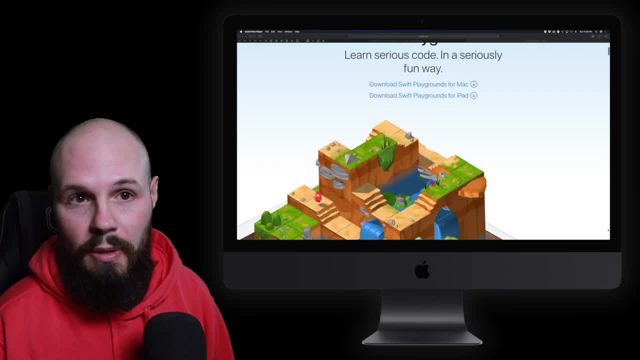 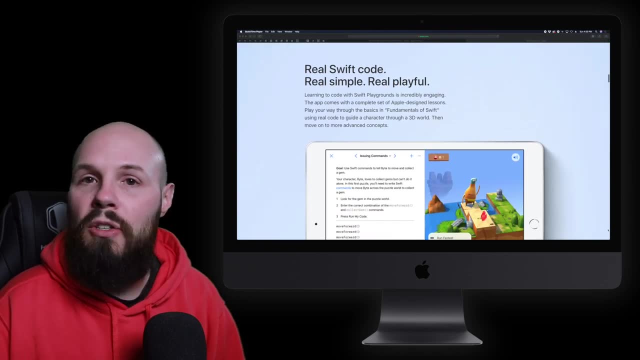 What is geared towards beginners is the Swift Playgrounds app, And I definitely recommend downloading that. It's free to download. It came out a couple years ago And it's being actively maintained. Like every year or so, you'll see a pretty big update to the app that adds a bunch of new features. 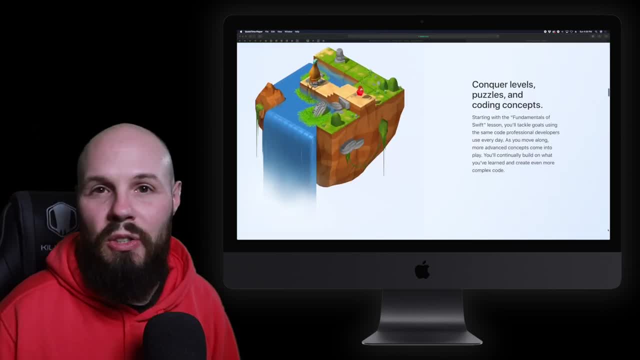 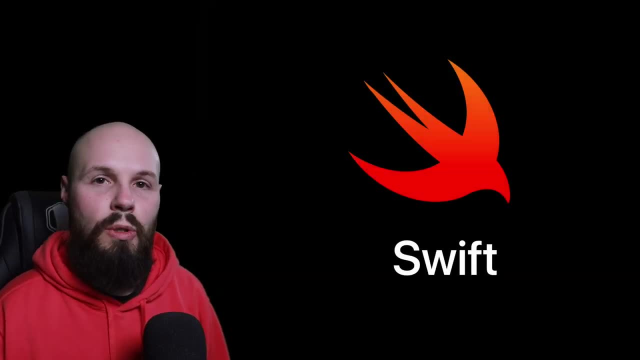 So that app is still growing, But that's a great way to get started and play around as well. They do a good job of gamifying things And in the description to this video I'm going to leave two more links. One is to the actual like Swift website page. if you want to check that out for another big overview. 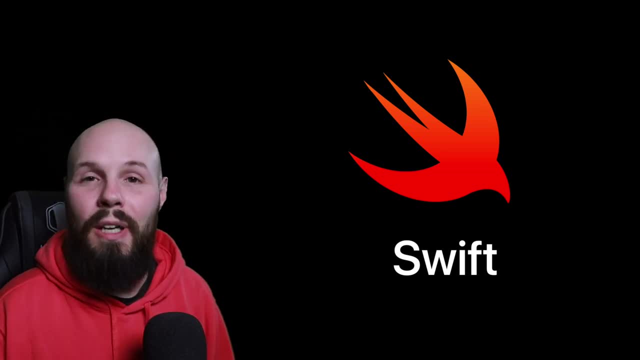 And then another is a pretty fun video about the review, A pretty fun video about the reveal of Swift at WWDC in 2014.. And you can hear like the gasps in the audience. It's pretty cool to go back and watch. 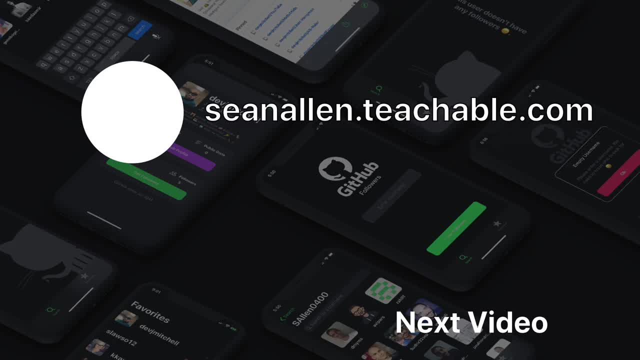 So that's a brief history of Swift. Let's start writing some code.